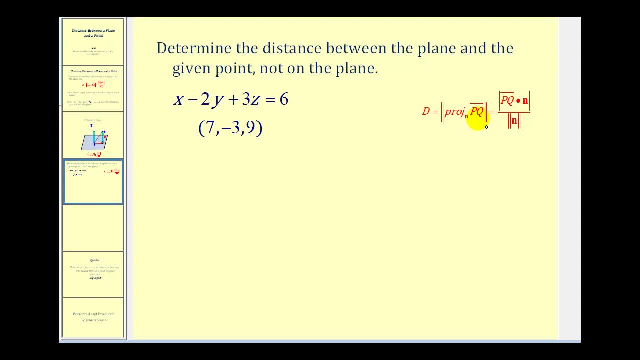 find the component form of the normal vector as well as the component form of vector PQ, where P is a point on the plane and Q is the given point. Let's start with the normal vector. Remember when we talked about the equation of a plane. the coefficients of the x, y and z terms give us the component form of the. 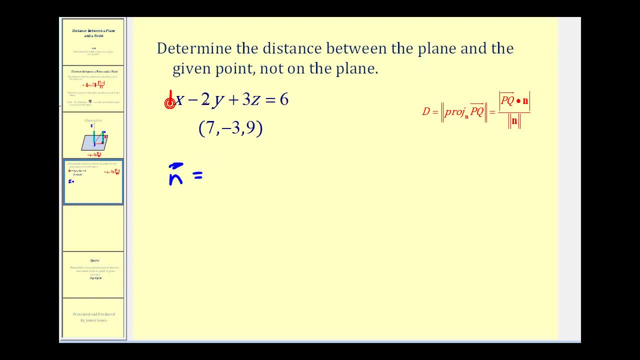 normal vector. So since the coefficient of the x term is one, the coefficient of the y term is negative two and the coefficient of the z term is positive three, the normal vector will be the vector with components one, negative, two and positive three. Now we need to find the component form of vector. 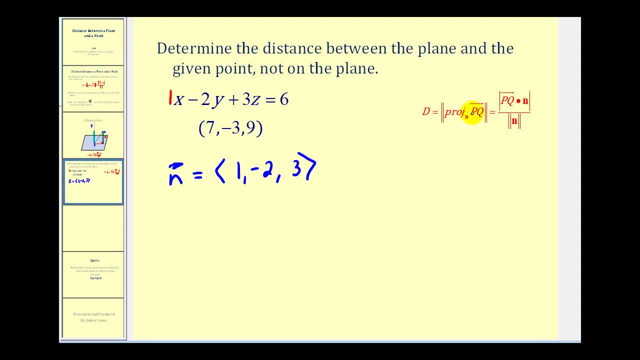 PQ. Remember, P must be a point on the plane and we're not given a point on the plane, so we do need to find one point on this plane. So for point P, if we let x equals zero and y equals zero, we would have the equation three z equals six, which means 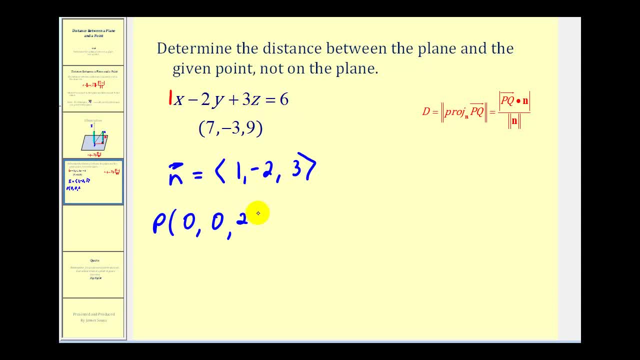 the z coordinate must be two, So we'll use this point as the point on the plane. of course we could use any point, but this one's convenient, and then point Q will be the given point, seven negative three nine. So now we need to determine. 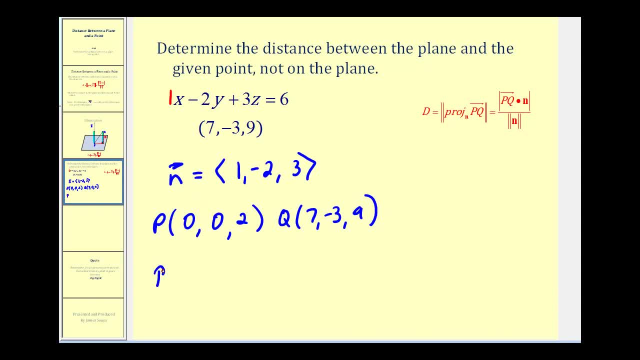 the component form of vector PQ. So that'll be seven minus zero, negative three minus zero and nine minus two. Now we have all the information we need to determine the distance given by the absolute value of the dot product of the two vectors divided by the magnitude of vector n. So let's go ahead and figure out what that. 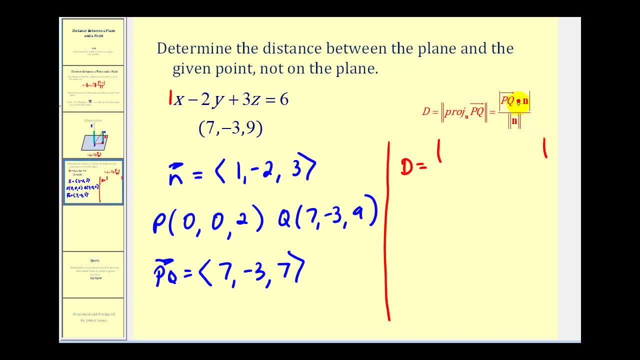 would be. So we're going to find the absolute value of vector PQ dotted with vector n, So we'll have one times seven, that'll be seven plus negative, two times negative three, that's six plus three times seven, that's twenty-one divided by the.